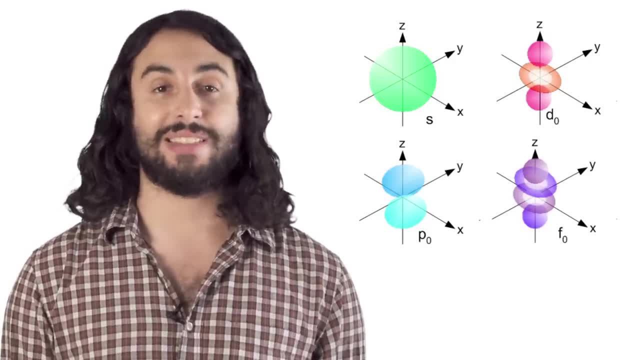 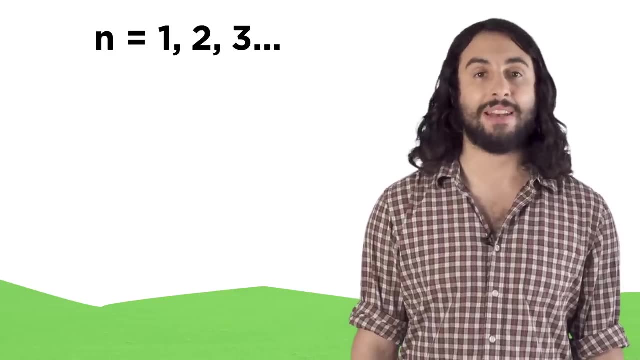 one can hold up to two electrons. The more electrons an atom has, the more of these orbitals it will need to accommodate them all. The first quantum number is the principal quantum number, n, which can have any positive integer value. We saw this when we learned about the. 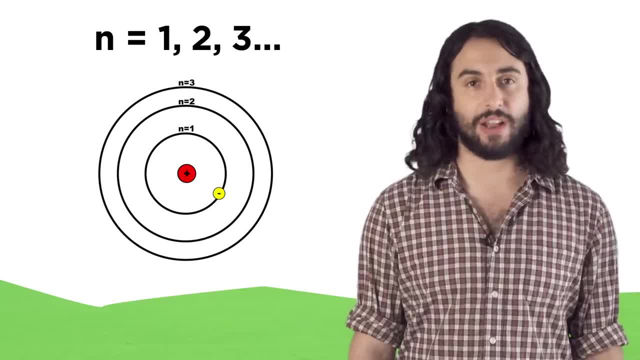 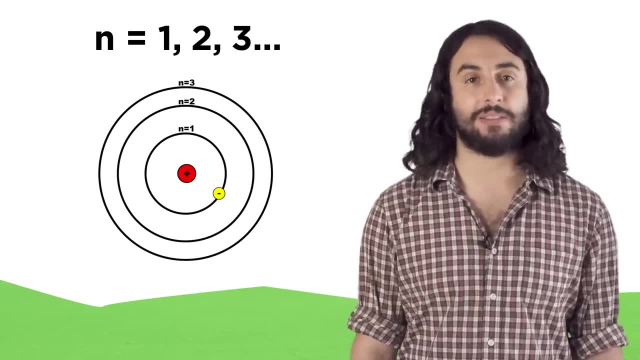 Bohr model. It represents the energy level of an atom. Each orbital will have an n value and the larger the value of n, the further away from the nucleus it is. The next quantum number is the angular momentum. quantum number l. 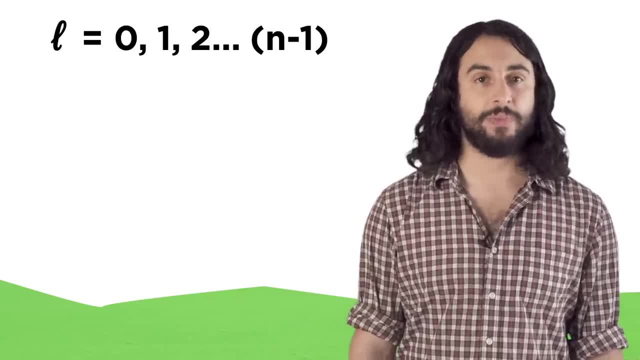 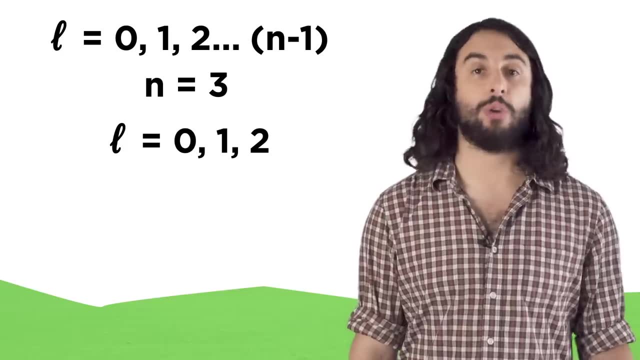 This can have any value from zero to n-1.. For example, if an electron has an n value of 3,, it can have an l value of either 0,, 1, or 2, because 2 is 3-1.. The l value describes: 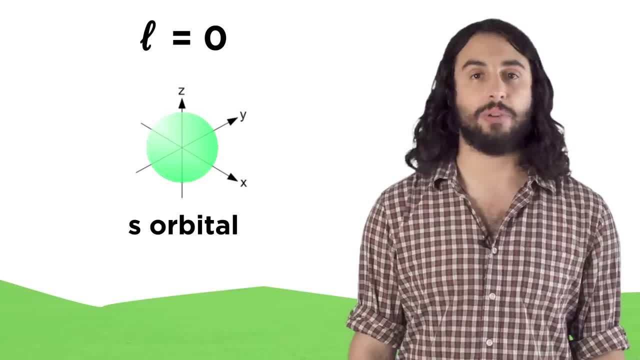 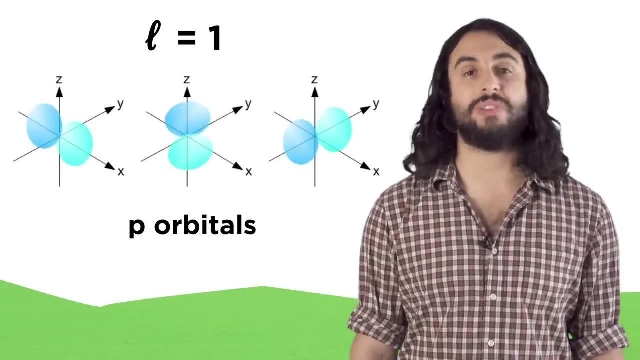 the orbital. When l equals 0,, we are describing s orbitals, which are spherical, just one of these per energy level. When l equals 1, we are describing p orbitals, which are lobes that extend outwards on three axes. There are three of these per energy level. When 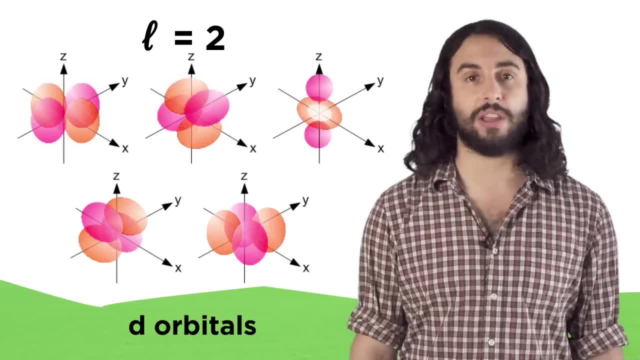 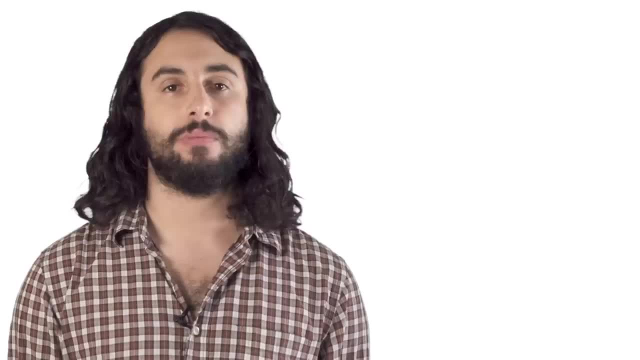 l equals 2, we are describing d orbitals, which are weird looking, five of these per energy level. And when l equals 3, we get f orbitals, which are even weirder looking: seven per energy level. Next, we have the magnetic quantum number m sub l. This 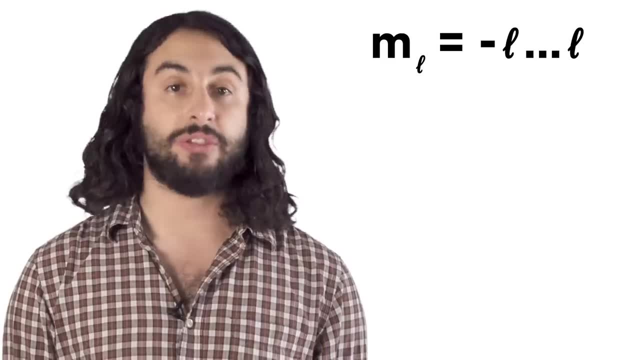 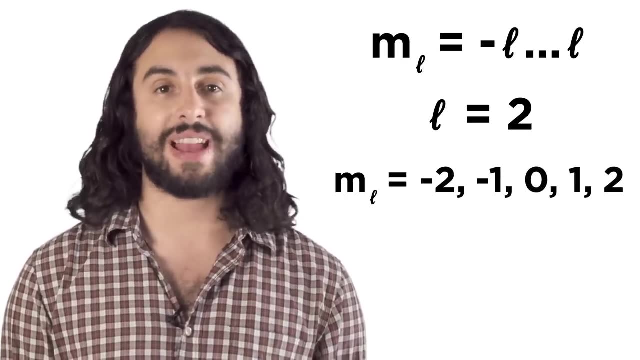 can have a value of anywhere from negative l to l. So if l is 2, m sub l can be negative 2, negative 1,, 0,, 1, or 2.. This quantum number determines how many orbitals there are of. 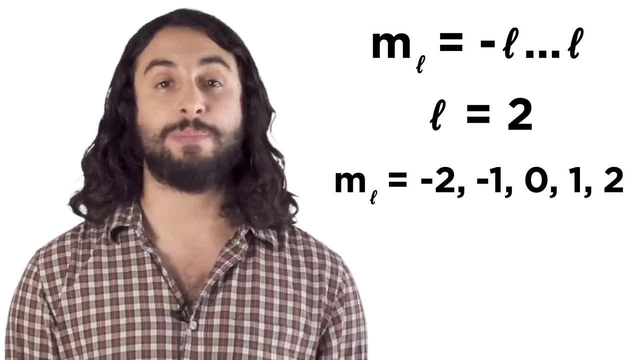 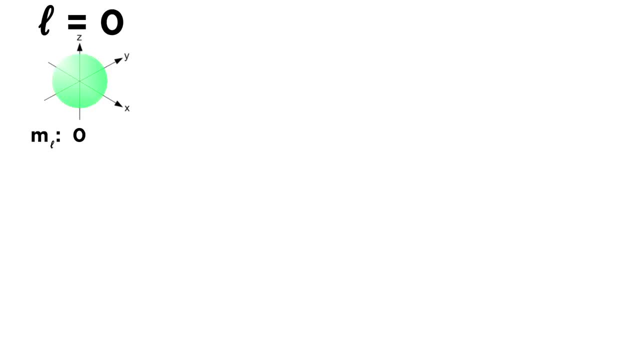 a type per energy level and therefore describes a specific orbital amongst a particular set. When l is 0, m sub l must also be 0, and that's why there's only one s orbital per energy level. When l is 1, m sub l can have three values, which is why there are three p orbitals. 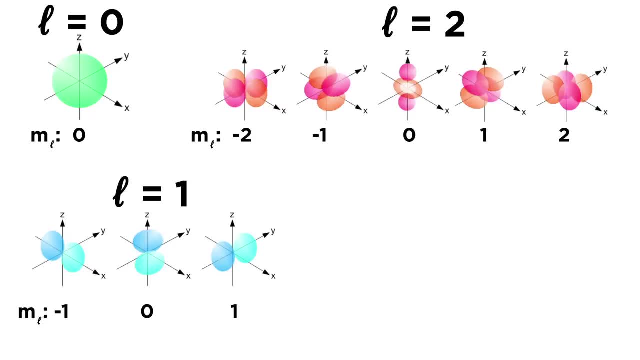 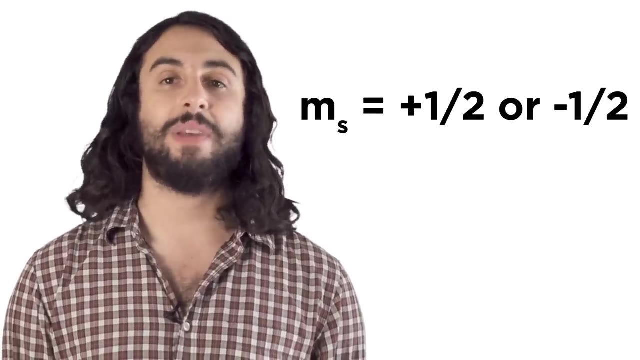 per energy level. An l value of 2 gives us five values for m sub l and five d orbitals, and an l value of 3 gives us the seven f orbitals. The last quantum number is an easy one. it's the spin quantum number, m sub s. This one will be either one half or negative one half. 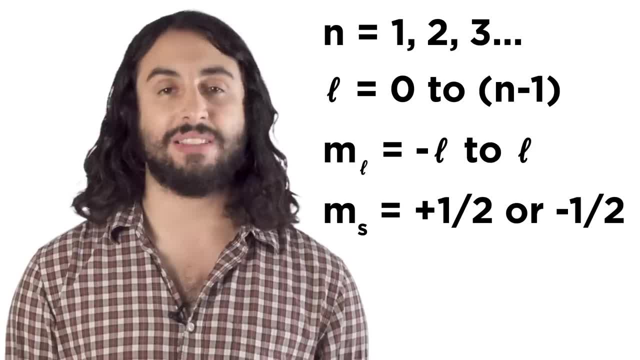 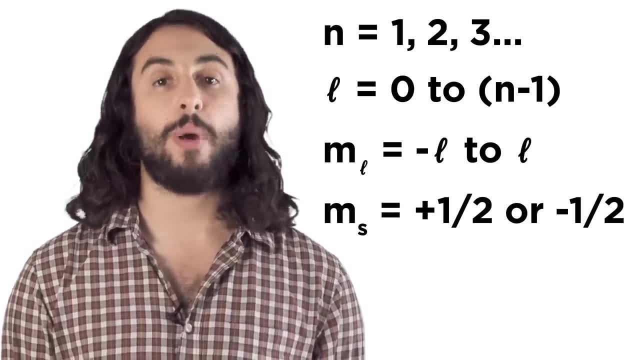 no matter what. So every electron in an atom has a unique set of quantum numbers. No two electrons in an atom can have precisely the same four quantum numbers, as is stated by Pauli exclusion principle. This is because any orbital can only hold up to two electrons. 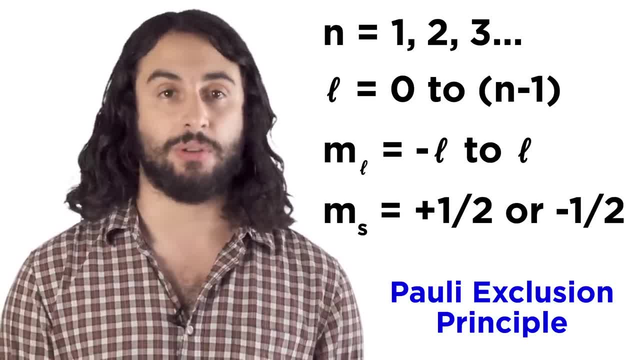 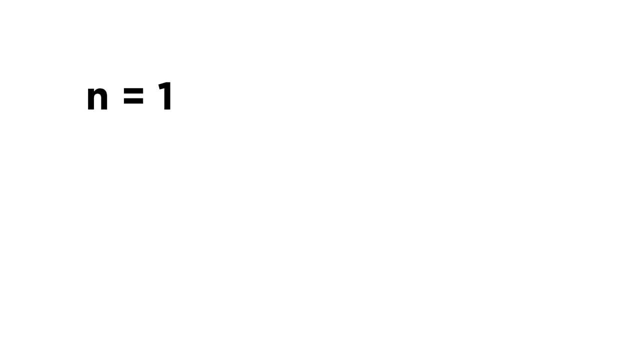 and even the two electrons in the same exact orbital will have opposite spin values. So let's try to describe different sets of quantum numbers and what they mean. When n equals 1, l must be 0, and m sub l must also be 0. That means we are describing the one s orbital. 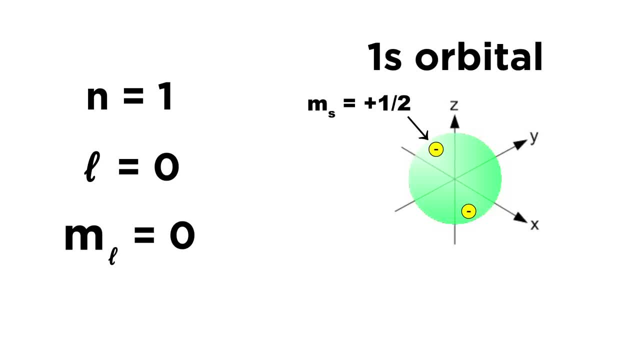 It can accommodate two electrons which will have spins of half and negative one half respectively. This is the lowest energy orbital, so any atom on the periodic table will fill this orbital first. The electrons in hydrogen and helium occupy this orbital, since they 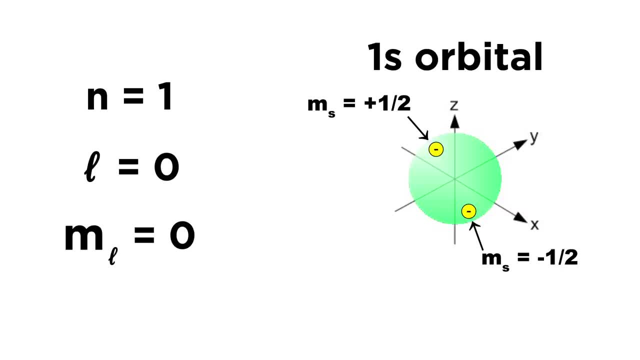 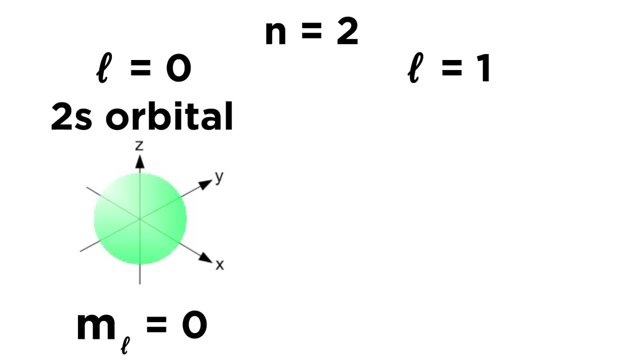 have only one and two electrons respectively. When n equals 2,, l could be 0,, which would give us the two s orbital, or l could be 1,, meaning m sub l could be negative, one zero or one, giving us the two p orbitals, The outermost electrons in the second row of the 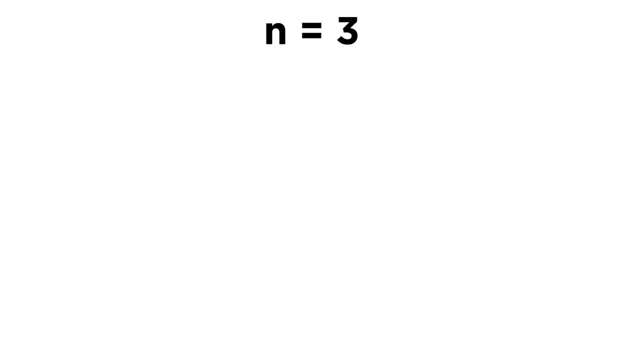 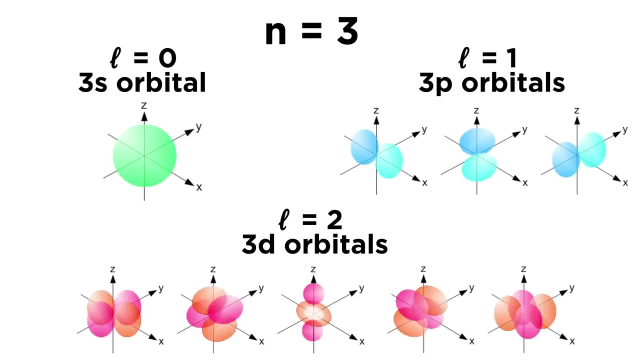 orbital will occupy these orbitals. When n equals 3,, l could be 0,. giving us the three s orbital, l could be 1,. giving us the three p orbitals, or l could be 2,. giving us the three d orbitals, A large atom will have to use all of these orbitals and more, to house. 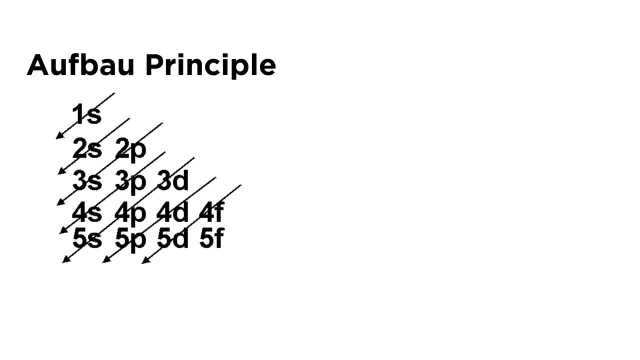 all of its electrons. The Aufbau principle tells us the order in which an atom will fill up its orbitals. This is determined by their relative energies. Orbitals that are further away from the nucleus are called orbitals. Orbitals that are further away from the nucleus. 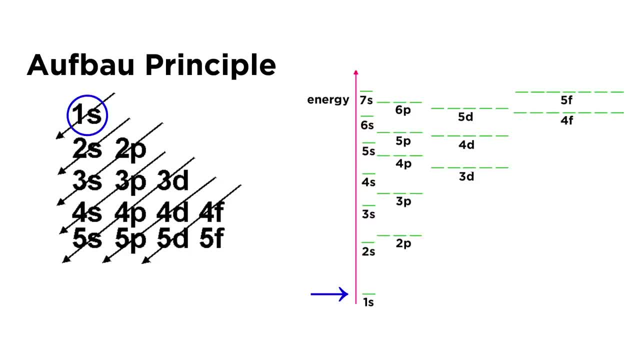 have higher potential energy. so it'll be 1s first, then 2s, then 2p, 3s, 3p and so forth. We can use this to determine the electron configuration of any atom, For example a. 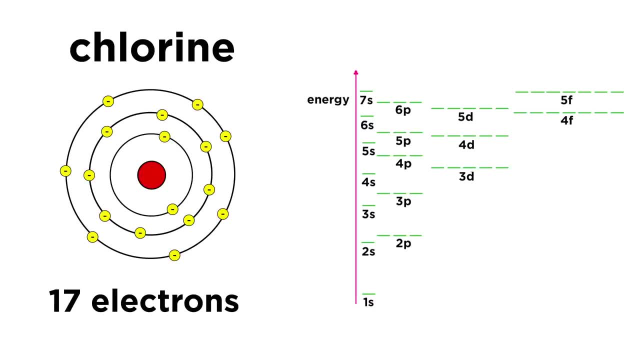 neutral chlorine atom has 17 electrons. so looking at the orbitals, each of which can hold two electrons, let's fill them up, starting at the lowest energy, and then climb upwards. The 1s orbital gets two electrons, one spin up, the other spin down, Then the 2s, then 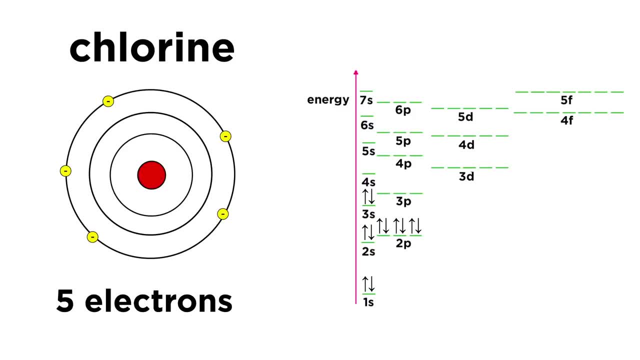 the 2ps, then the 3s and the last five will go in these three p orbitals. Hund's rule says that for electrons of the same energy you put one electron in each orbital first before doubling them up. So 1, 2,, 3, 4, and 5 gives us a total of 17 electrons. for chlorine, 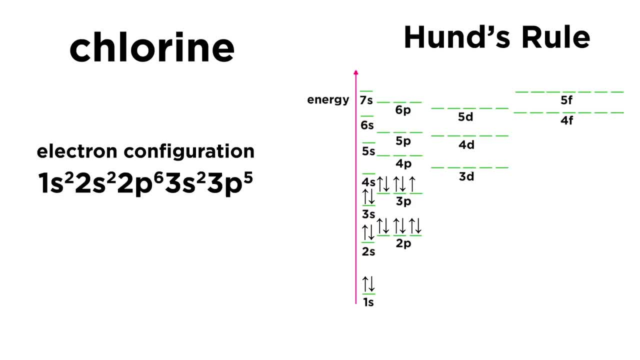 That means chlorine has an electron configuration of 1s2, 2s2, 2p6, 3s2, 3p5.. The numbers before the letters are the n value for the orbital. the numbers after the letters tell you how. 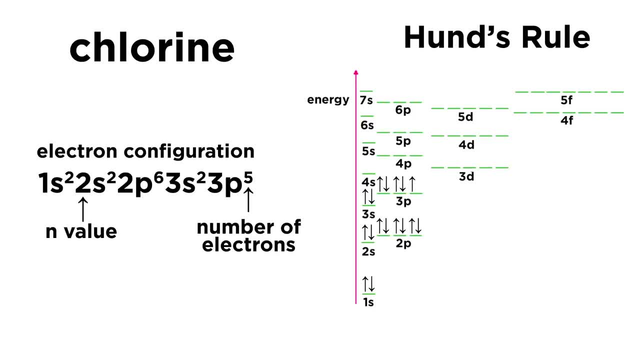 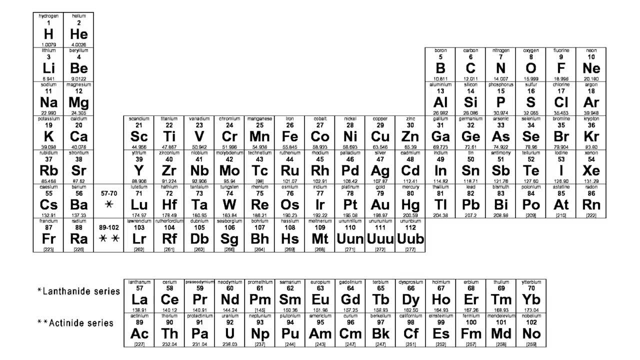 many electrons sit in each type of orbital. If you want a quicker way to determine electron configurations, just know which areas of the periodic table correspond to which types of orbitals. This area is called the S block, This is the P block, here's the D block and then the F block. When we are determining 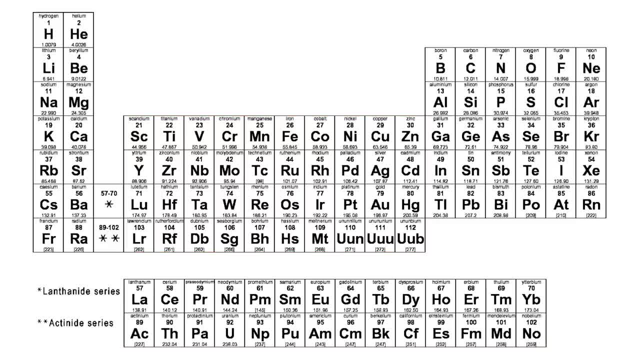 the electron configuration for an atom of a given element. the easiest way to do it just travel left to right and up to down on the table until you get to the element, since each element has one more electron than the last. looking at chlorine again, the top row is just the 1s orbital. that's full, so 1s2.. going to 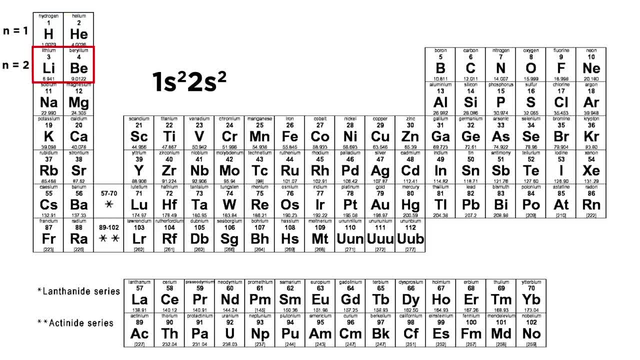 the second row, where n equals 2, we fill the 2s orbital, which holds two electrons, hence two elements, the two p orbitals which hold six. so we pass six elements, then the next row down, we fill the 3s orbital and, lastly, we get to the 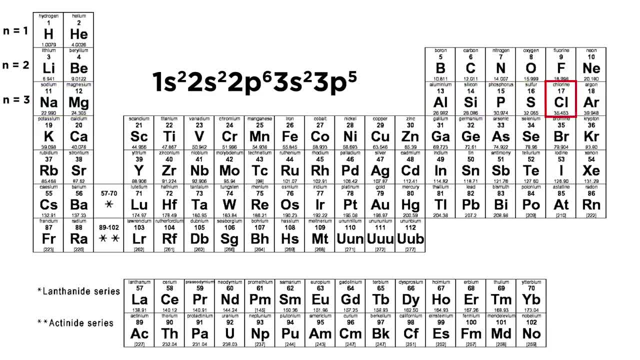 3ps and count one, two, three, four, five, 3p5.. a common abbreviation is to use the noble gas from the row above and list it in brackets. this would be read as neon core and it implies the ground-state electron configuration of neon. then you 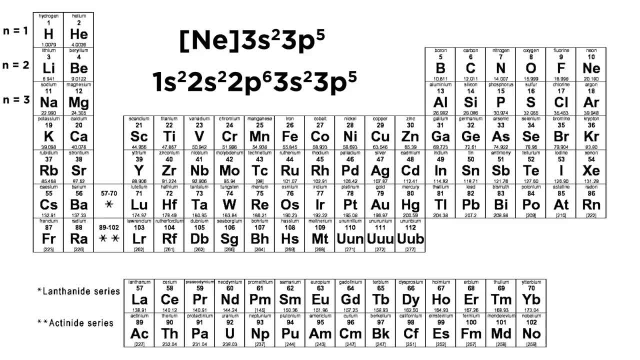 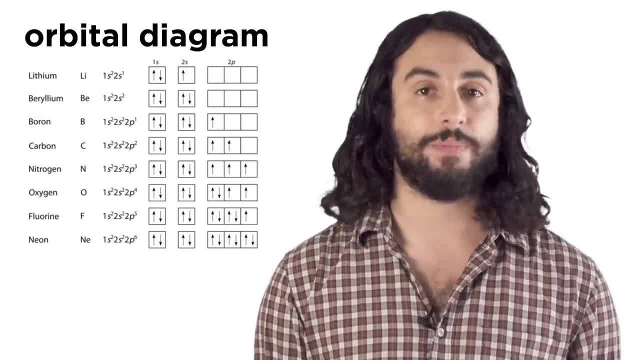 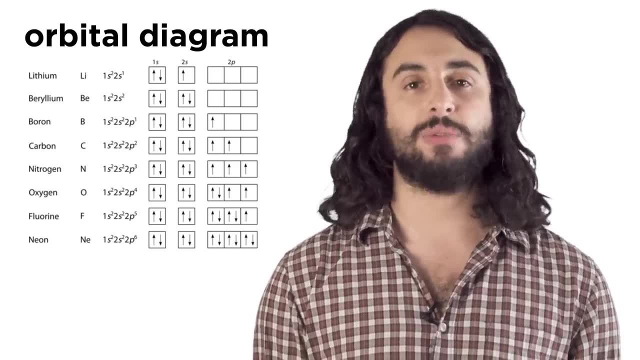 just list the valence electrons of the element or the ones that correspond to the row it is in. we can use orbital diagrams to visually depict how the orbitals are filled, and they look like this. don't forget Hund's rule: fill each set halfway before doubling up. for a quick definition: atoms with unpaired